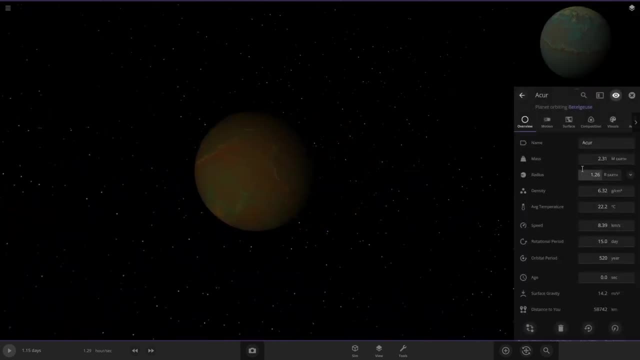 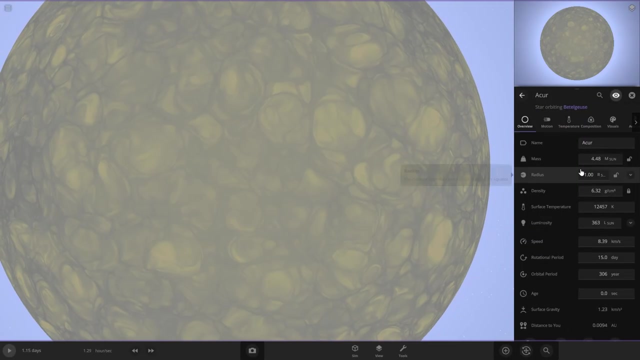 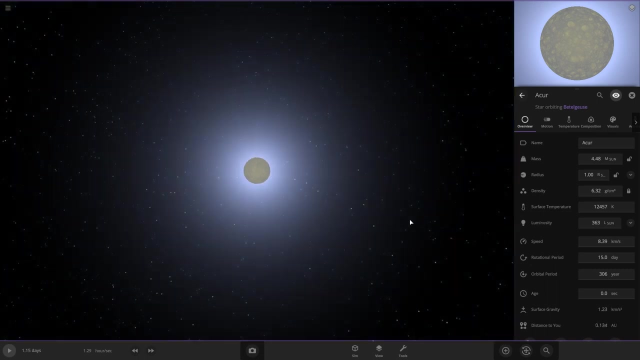 going to be big enough. We're going to need this a lot bigger. So if we just try to make the radius here, this is how big it actually is. If we just type one sun, it turns into a star, because the density is so strong that the gravity explodes in on itself. so that's not going to work. So let's. 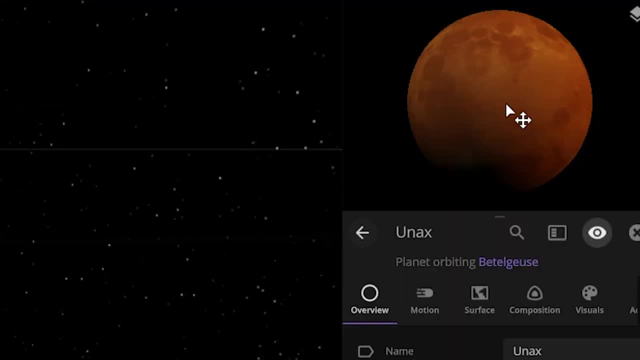 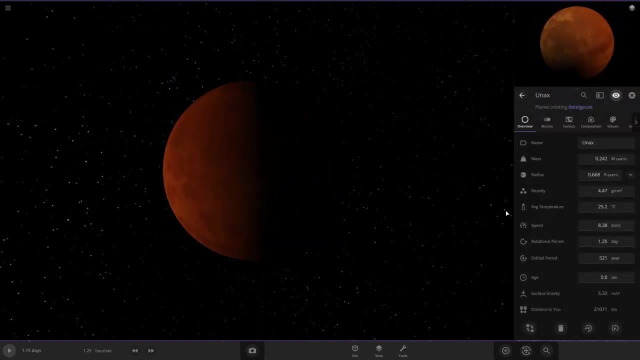 delete that And let's put a new planet in here. I like the way that one looks, So let's use this one, And I think that if we turn the density down, it should allow us to make it very, very large. So if we 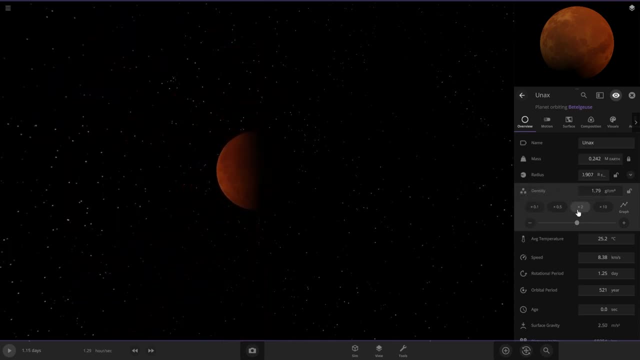 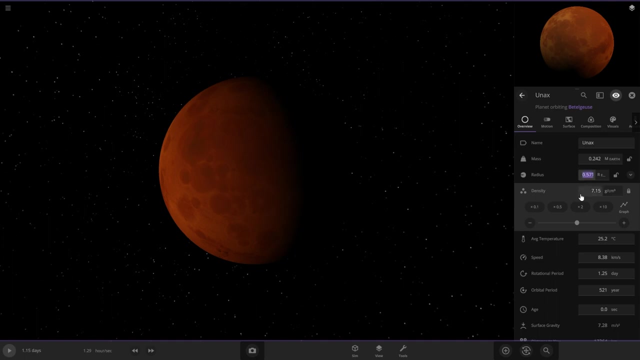 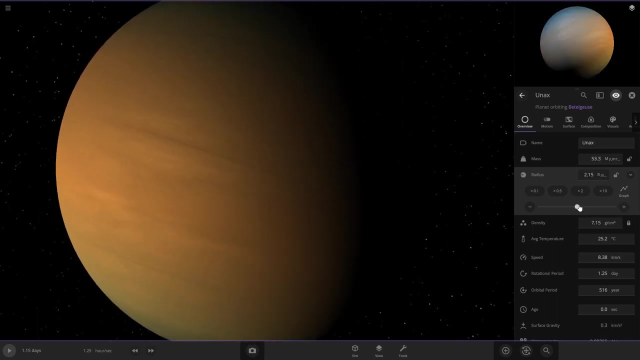 actually make it. So what we can actually do is find a good density, and if we lock the density like here, then when we turn the radius up it'll change the mass too. So it should stay at a good density where it's not going to, Okay. so it went to a gas. 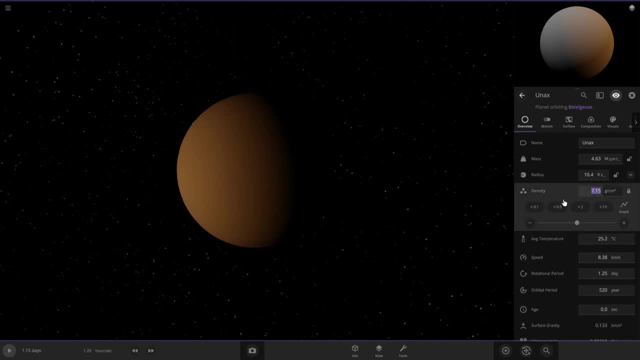 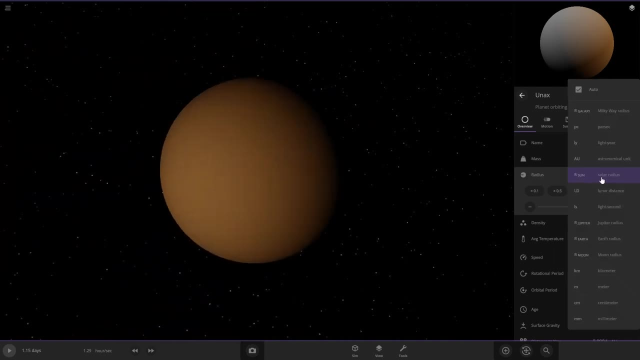 All right. so that means it's not light enough. So the density- if we just make this like ridiculously not dense and Oh, Oh, we did it, Okay, so right now this planet is 4.43 times the. 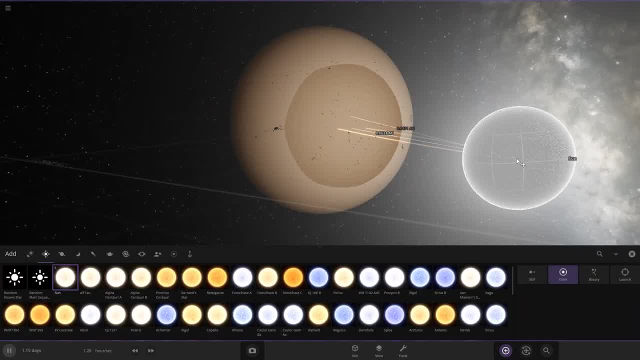 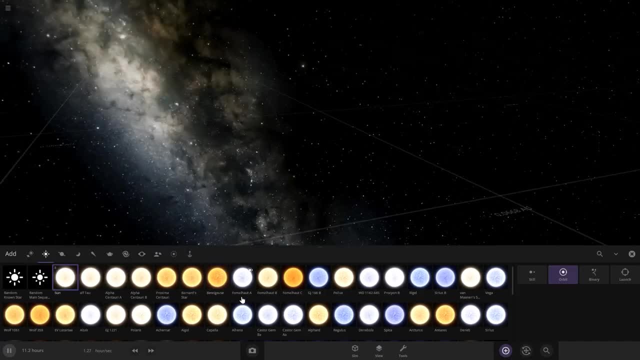 radius of the sun. So if we pull up the sun here, we can see it worked. Oh okay, something just happened. It just collapsed in on itself. Let's try it again. And because the planet's going to be so light anyway, I'm going to actually try to use the sun to see if we can get a. 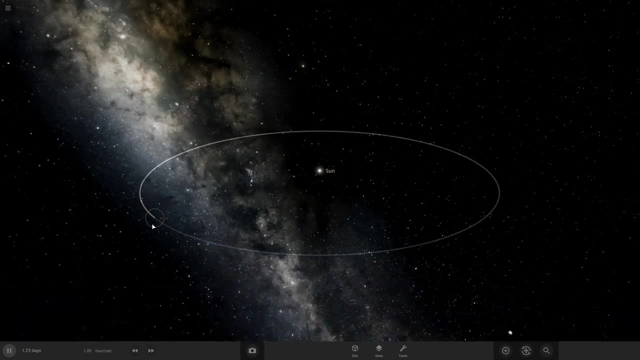 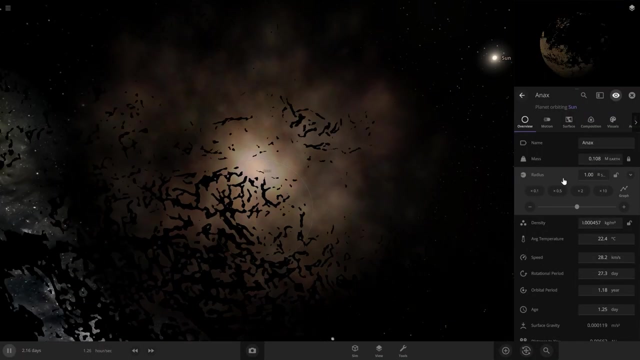 planet that looks very massive in its system. Okay, so we got another planet here. Put the radius very small, Small, can I do it? And then if we go to solar radius and then put one, And that didn't work, 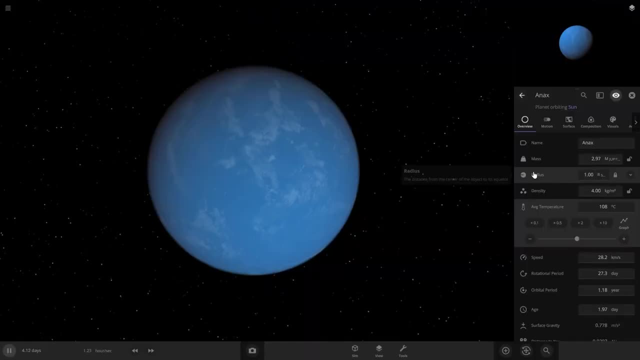 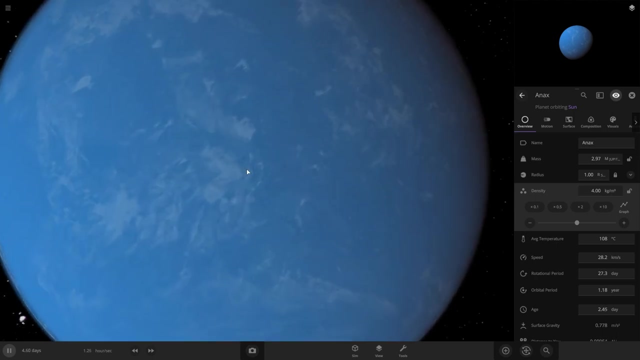 I locked its radius on one sun, so it will not change its size, And then I simply just made it less and less dense until it turned into a planet, And this actually looks pretty good here. already We checked the stats. We got a 6% Earth similarity, so that's not great. So 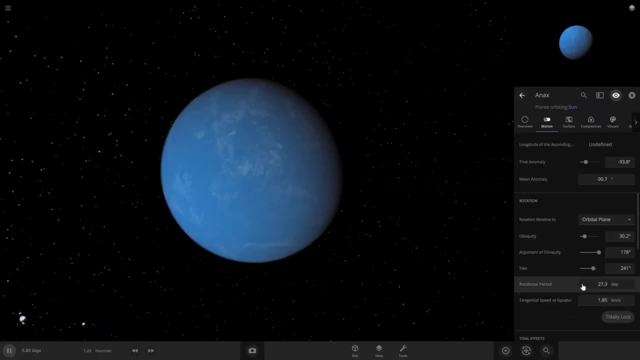 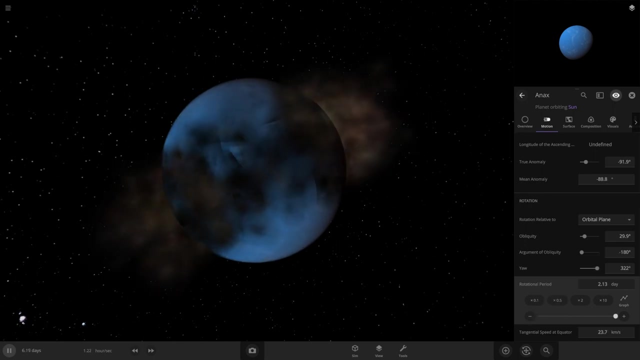 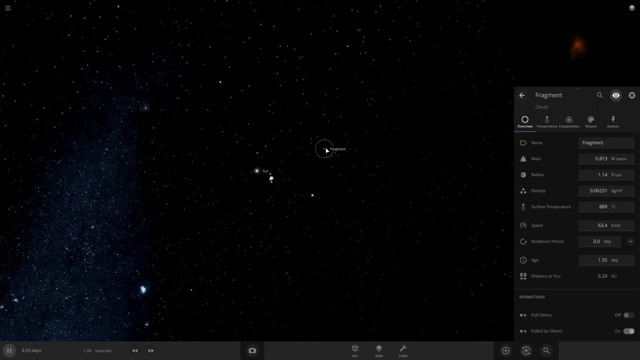 its orbitable period is about a year, which is what we want And our rotational period. We're going to want this a lot faster, so let's put it at one day. Oh, okay, so apparently it can't spin that fast or it shoots off stuff, So we're not going to be able to make it spin that fast. 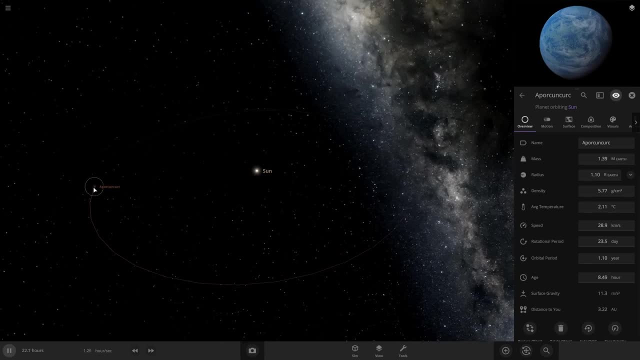 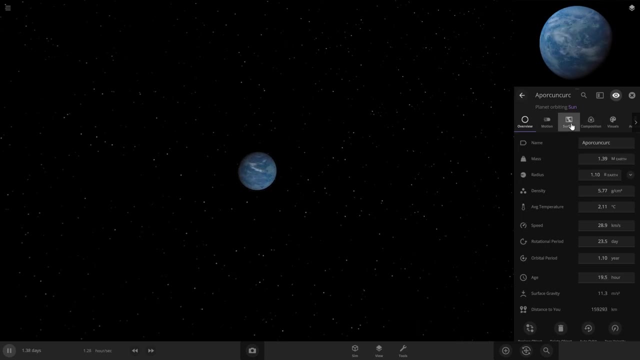 Let's try it again. So I guess, because it's so big, when it spins that fast, it shoots mass off of the surface because of the force, the spinning force. So we're actually going to want to change our rotational period right now. Let's put it at one year, just so it's tidally locked, which will make it not spin. 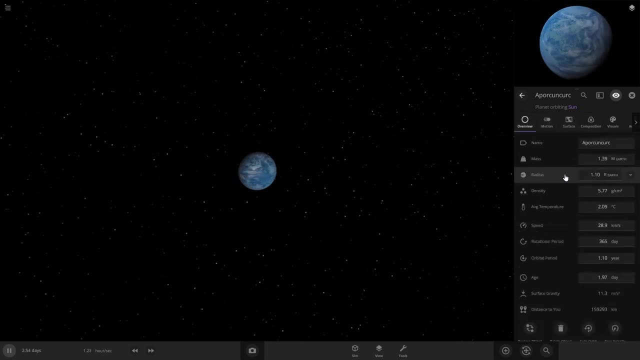 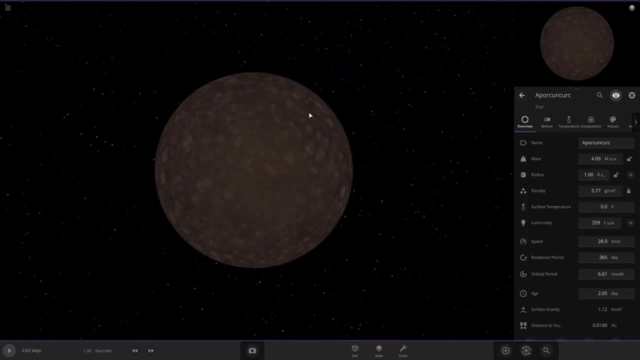 at all. So now what we can do is go back to the overview and we can lock If we pause time, so it doesn't change it right away. we type 1s for one sun And you can see it did turn into a star, but if we lock that, it's going to spin. So we're going to put it at one year, just so it's tidally locked, which will make it not spin at all. So now what we can do is go back to the overview and we can lock. 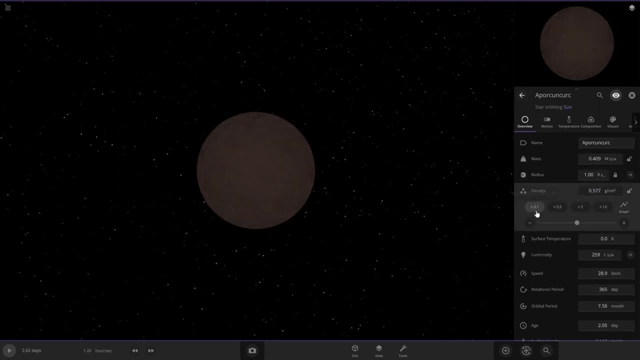 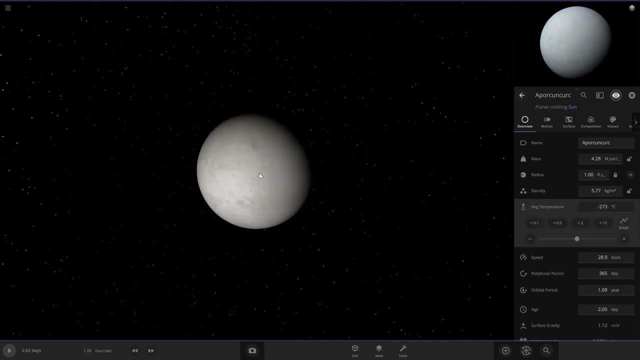 If we lock the radius, then turn our density by times 0.1. So that turned it into a gas giant. but we want it even less dense, so it'll go to a rocky planet like this. So now we do have a rocky. 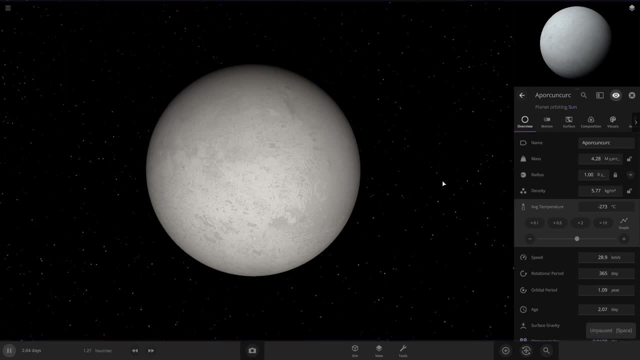 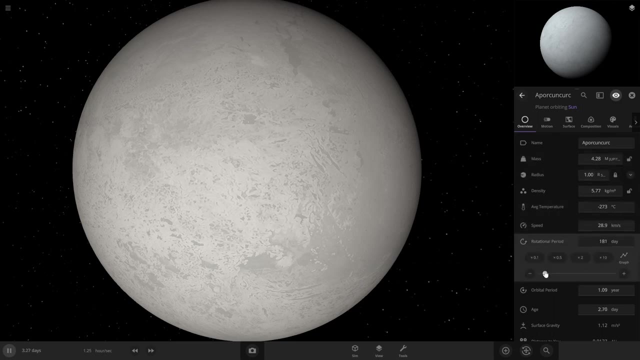 planet here. I'm worried that this is going to not be stable when I unpause it. Okay, so it looks like it's not going to just die, So I wonder how fast we can spin it without it shooting off fragments. Okay, 2.5.. I'm just going to leave it there, because once I went faster than that last. 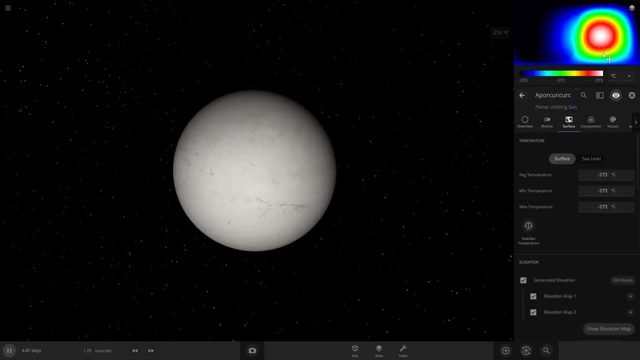 time it didn't spin. So I'm going to go back to the overview and I'm going to put it at one year, completely broke apart. So if we go to surface now, we can see that the hottest it's getting is. 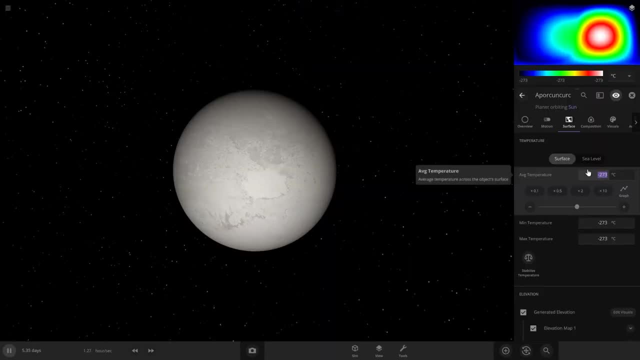 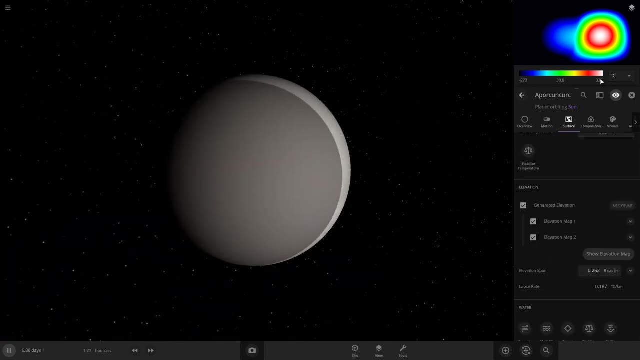 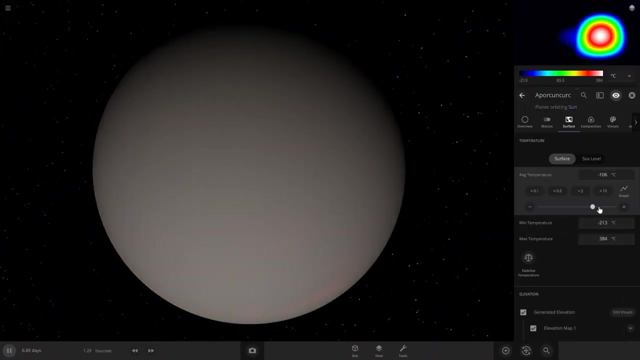 273. That's absolute zero. So let's change this to 30, just to see what happened there. One spot of it heated up, So it looks like now half of it is 335 Celsius and half of it is negative 273. So if I heat it up, it only heats up one side of it. What is this pattern? I'm 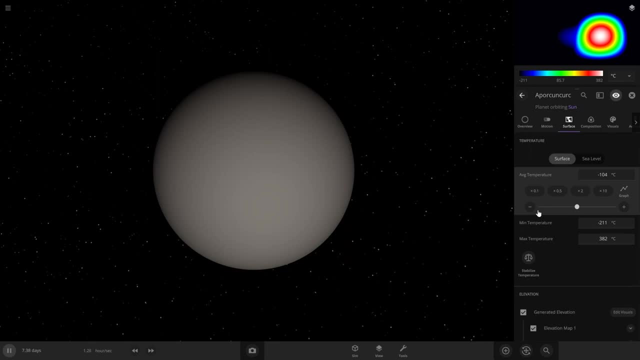 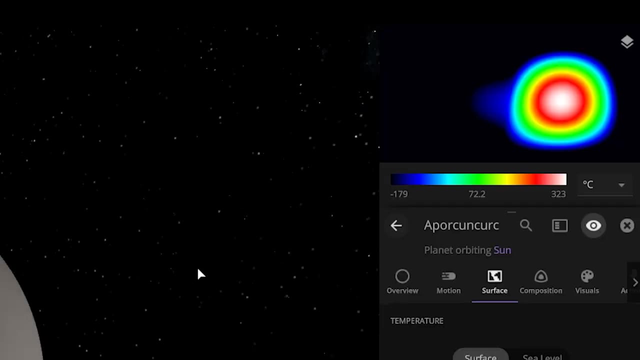 wondering if it's so big that the game doesn't know how to heat it all up evenly. So we want the average temperature to be around 25.. But the problem is up here. you can see on this graph that half of the planet is still very, very cold, which it also has no. 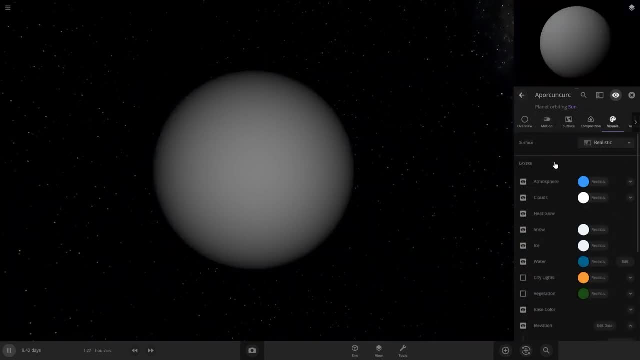 landmasses. So we can actually change that. because of the newest update, We can go to generated elevation here and click edit visuals and we can change it. But I think is it still a gas giant? Is that what it is? It's heating up. Oh, it's going to shoot fragments. 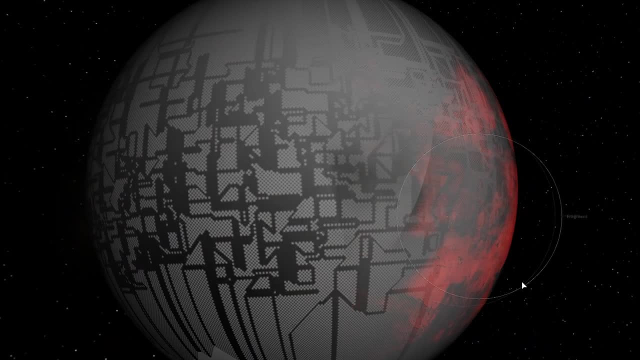 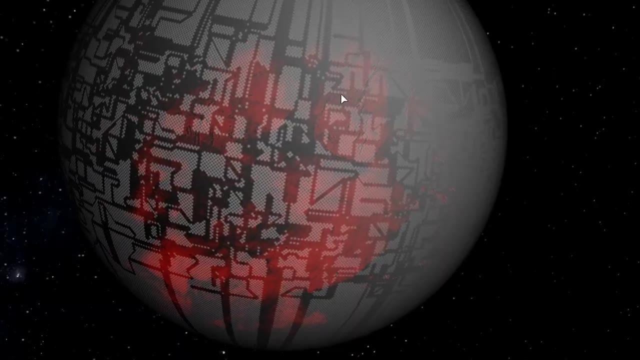 Okay, So now it's definitely a gas giant. Oh, my goodness, What did we do? This looks like the Death Star. I've never seen anything like this, And that is definitely a smiley face telling us we've done something very wrong. I actually want to save this object in this. 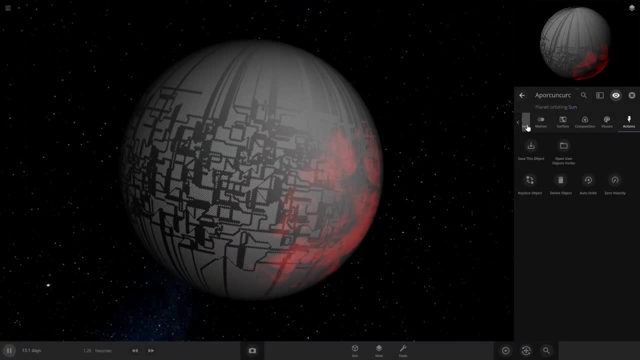 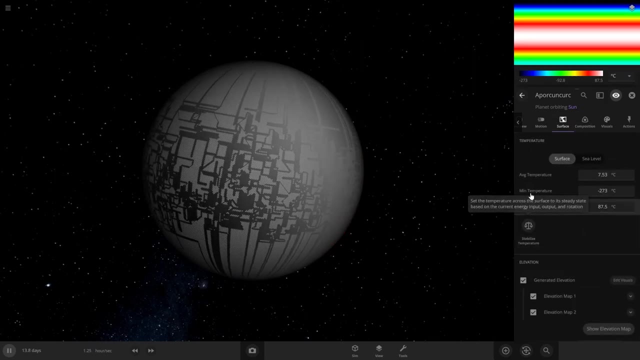 state to see if we can. let's name it Death Star. That is insane, Okay. Okay, Let's check out. I have no idea what, how to. okay, let's try stabilize temperature. Oh, that actually worked fairly decently. I mean, it's very cold at the poles, but we're going to ignore that for now. I kind of 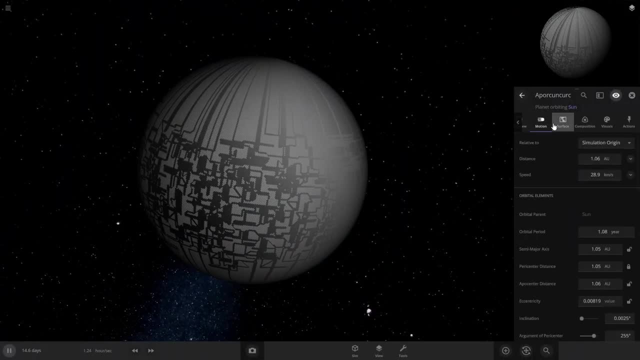 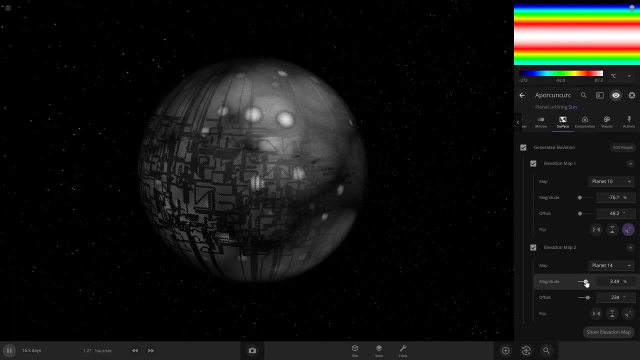 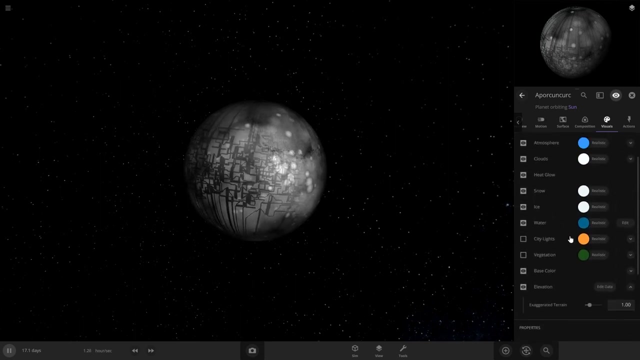 don't know how it looks, So let's see if we can get it habitable now. If we go to, I want to get a elevation map on here so we can steal it from Mercury or anything. Let's get it like about there And I'm not even sure what happened here. I'm going to try to switch the colors on it, So 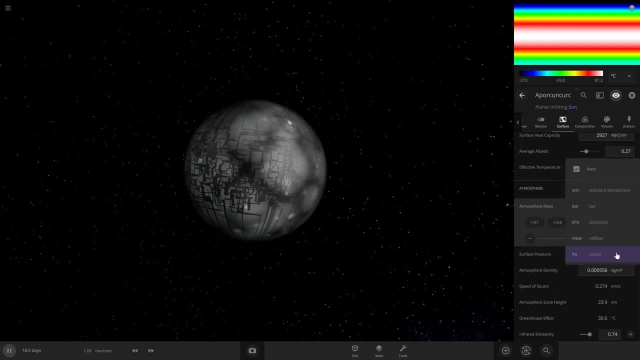 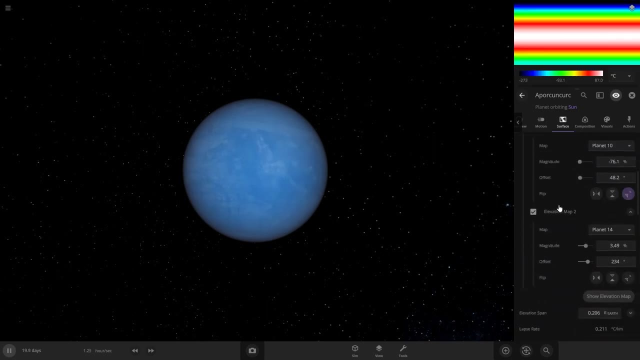 it does have an atmosphere right now, but I'm not it's going to need to be about one bar, Uh, and then we can actually make it. So it's not so thick. Let's do the water. Where's the water? 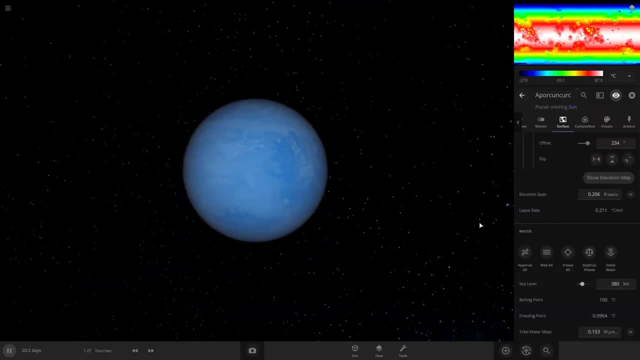 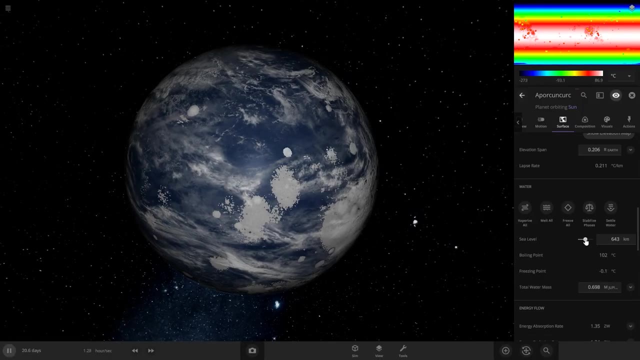 Sea level. Okay, So now we can get some water on the surface. You can kind of see it. Let's turn off the atmosphere. So we got water on the surface. We want it- mostly water- So let's do probably about there. Then I don't like how all of the land is just white, So I'm going to try to fix that. 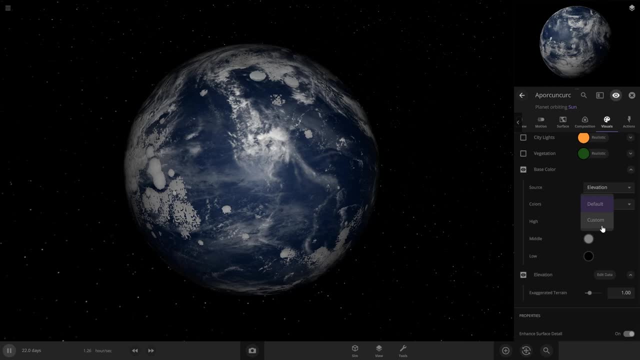 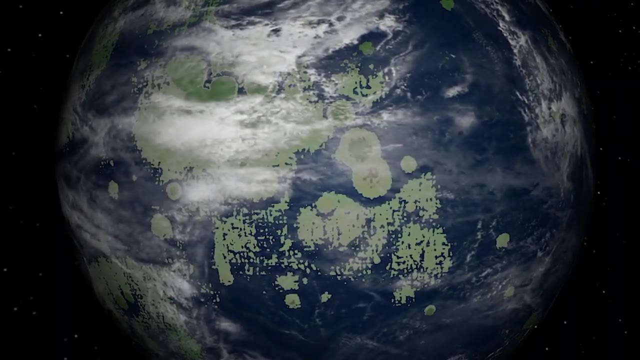 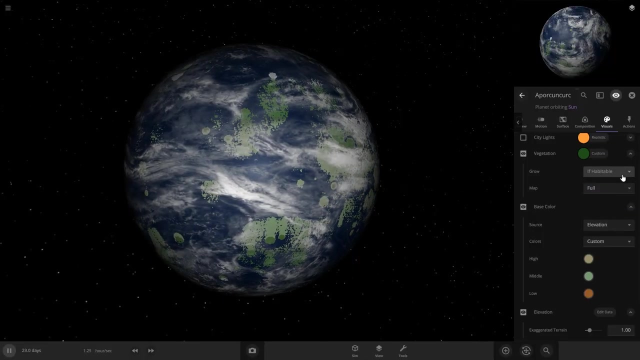 So it somehow defaulted to white, gray and black for the colors. So we're going to just switch that and we can do with the new update. We can actually add vegetation. Oh my goodness, See, look, grow if habitable map- or we could do, I mean earth- but we're just going to do full. That means 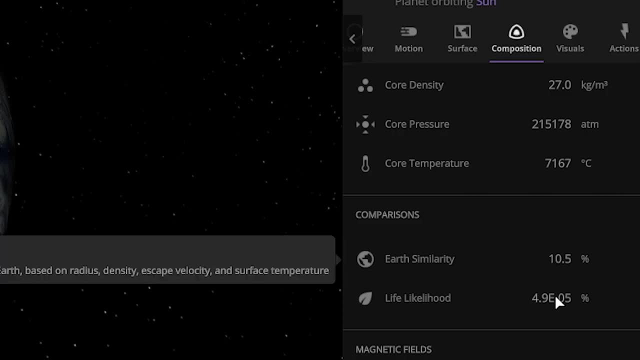 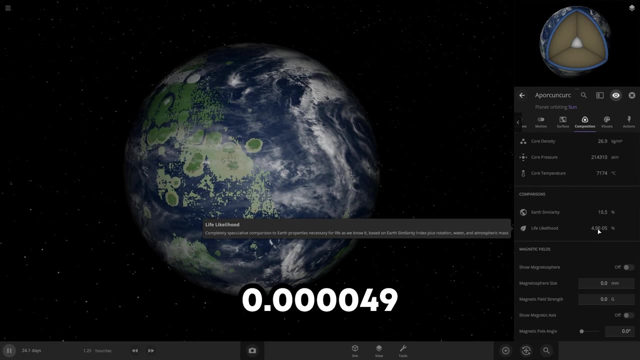 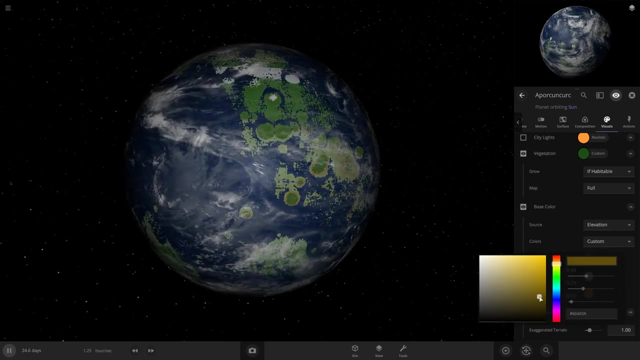 that this planet must be habitable. Yeah, So we got 10%, or similarity, and somehow we got 4.9 E to the negative fifth power, which is this number of percent life likelihood. So there's not a very high chance yet, So let's try to see if we can increase it. I want to set these to more of like brownish. 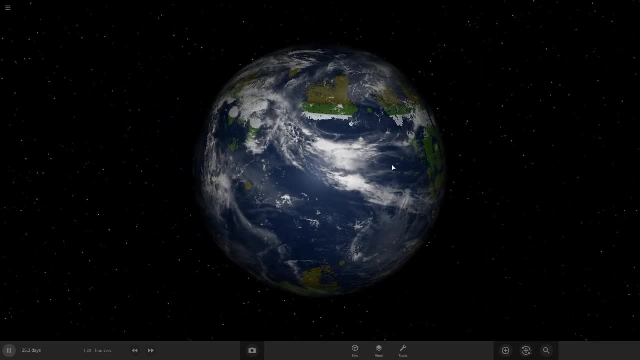 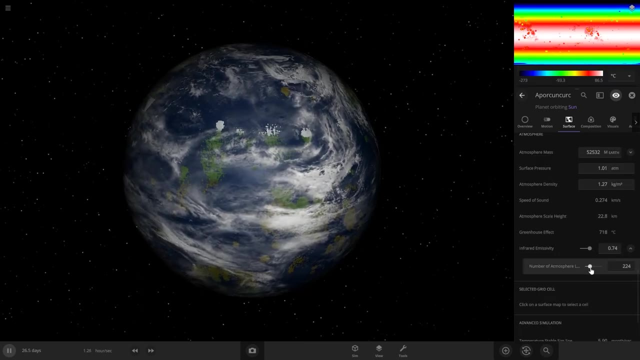 tones because we actually have the vegetation now. So what we can do now: try to heat it up a little bit more. Um, I'm going to add more atmosphere layers which can help with how much your planets gets heated. Let's try seven. We just speed up time. We'll see what happens. So this average.